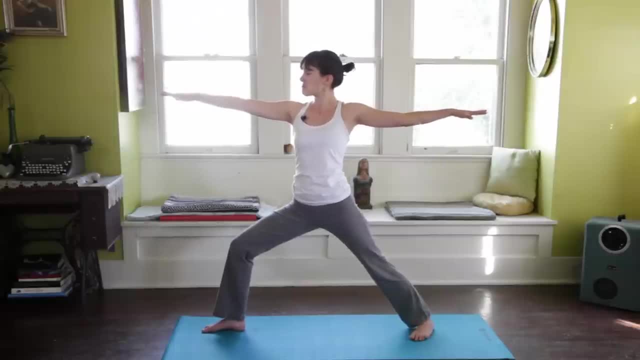 I bend my front knee And check out Warrior 2 today. Couple of action points, couple of alignment notes. I don't want this knee to go past my ankle. in fact I want it to be the shin, to be perpendicular to the earth and kind of create a nice right angle here. 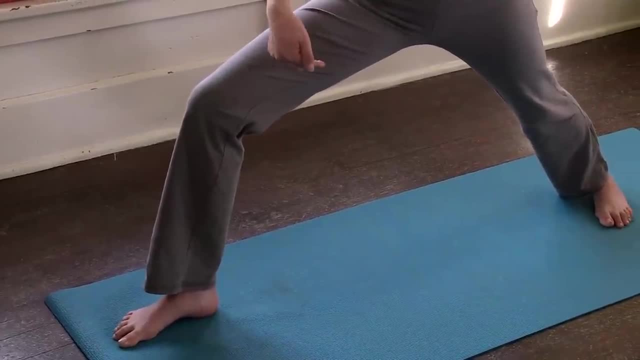 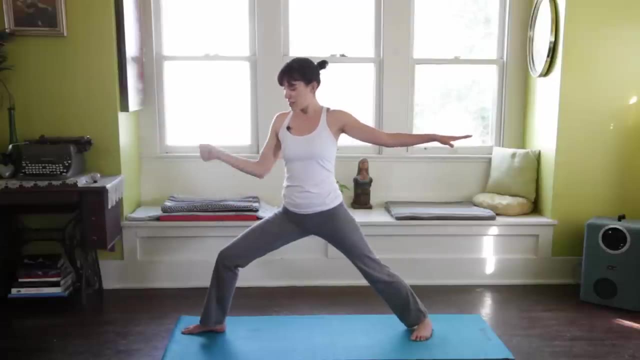 So I can walk my toes out if I need a little more space, or I can walk them in if I need to find more stability, but I want to get to a place where I can see my front big toe. So if the knee is coming in, which is going to be a tendency, I'm going to say no, thank. 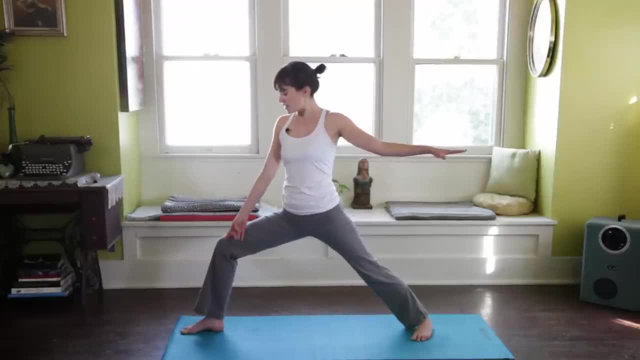 you mindful, bring it out and see if I can take a look down at my big toe Now. my right arm is extending out. excuse me, my left arm is extending out, nice and long. My right arm is going towards the front of the room. 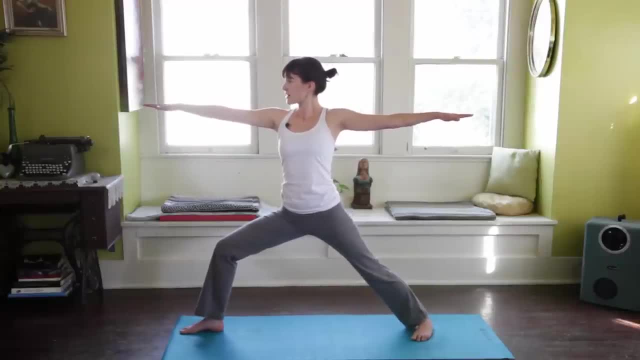 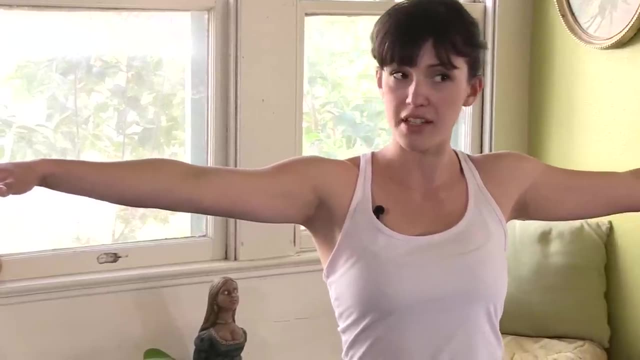 And then I just breathe here, check in, Maintaining the integrity of that back foot, maintaining the length in my spine As I get tired. this leg is going to want to unbend, but I'm going to sink in deep, breathing into my full torso. 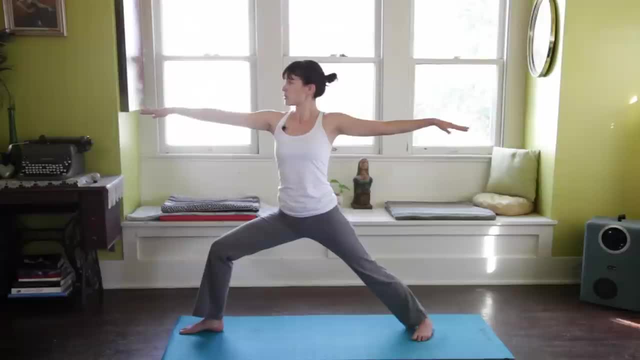 As I'm here, I can take a check into the shoulders by inhaling, opening the palms, wide, open heart, And then keeping this spiral in the shoulders and this open heart. I'm going to pancake the palms back down, but keep the shoulders where they are. 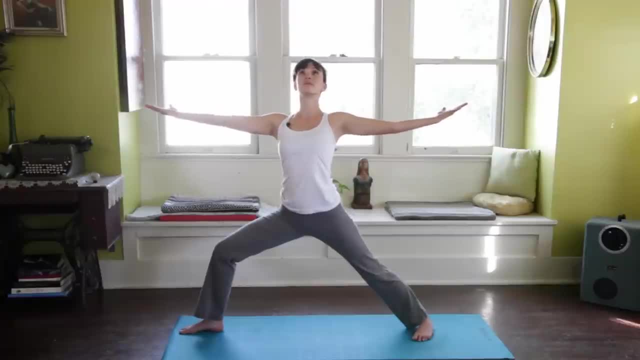 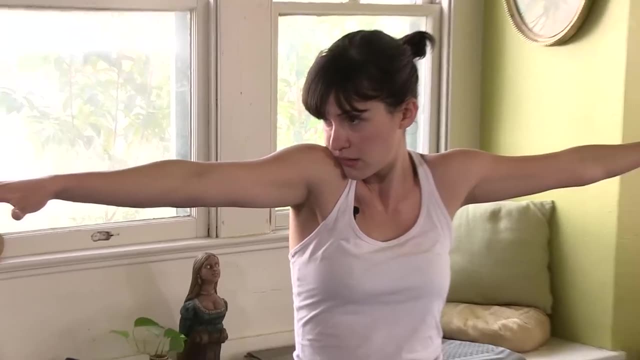 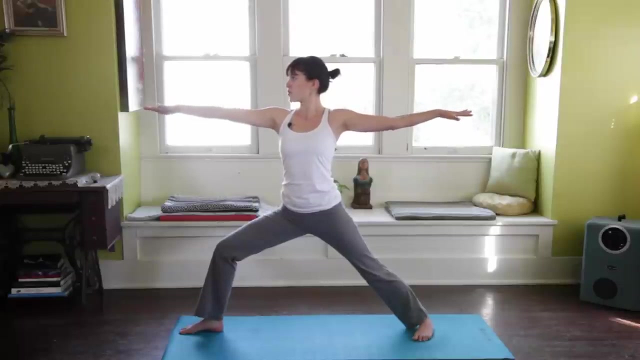 Can maybe try that again: inhaling, opening the shoulders and then turning the palms over. So I'm maintaining this nice open spiral of the shoulders rather than being here. That's an exaggeration, of course, But I'm creating a little space growing from there and then palms back down parallel. 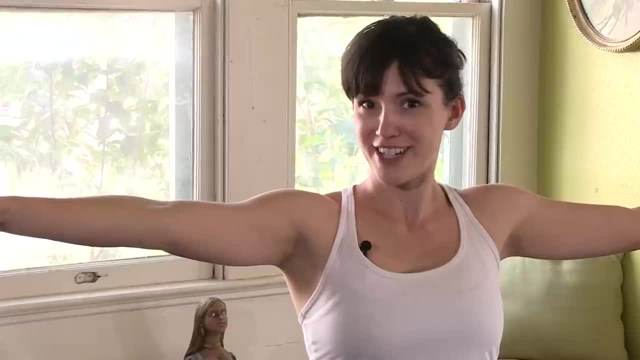 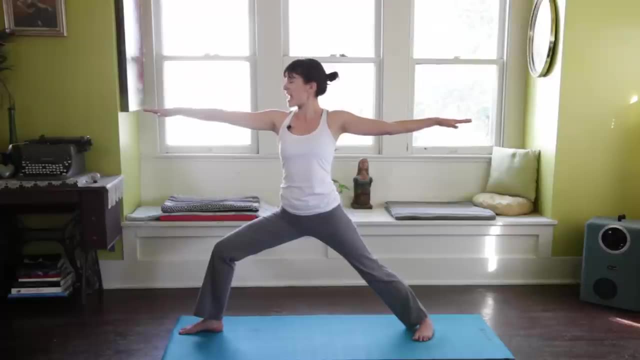 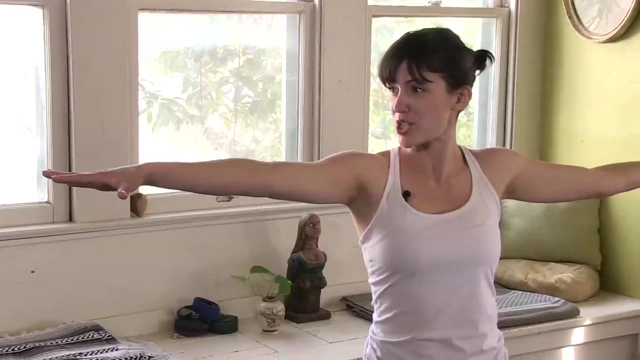 to the earth Again. no breath count again. today We're just breathing here. I just want to encourage you to breathe here, Drawing up through the arches of the feet, pressing into that outer edge of the back leg. Warrior, The mantra or the affirmation here is: I am strong. 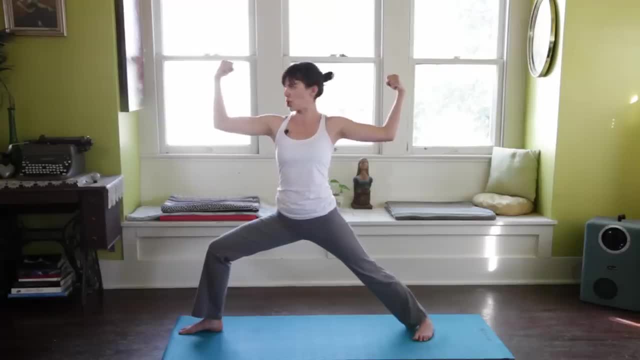 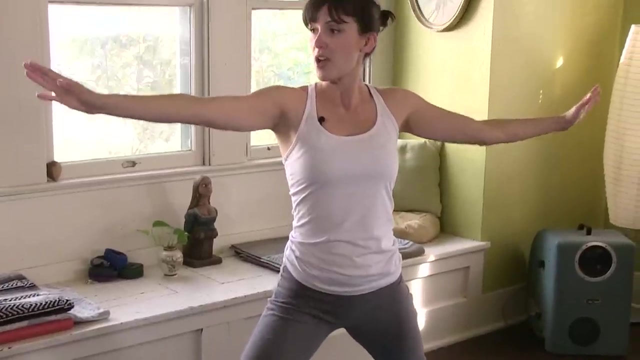 That's what we do in kids yoga. I am strong Warrior, Nice and easy in the face, strong in the lower body. Keep tucking that pelvis in And then, when you feel satisfied here, we'll inhale in, exhale. straighten that front leg.